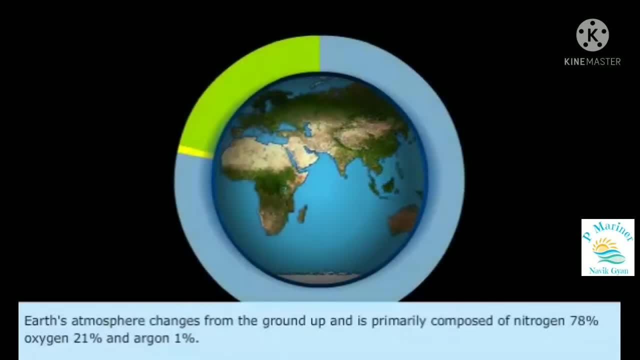 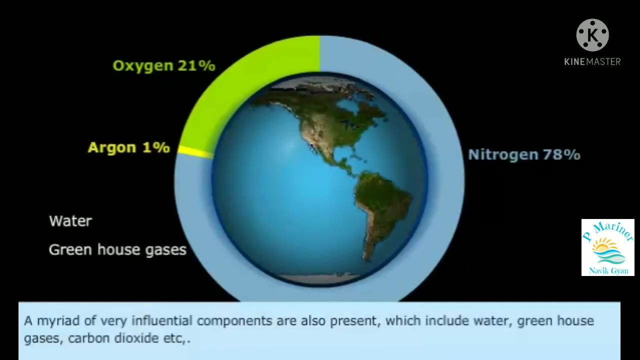 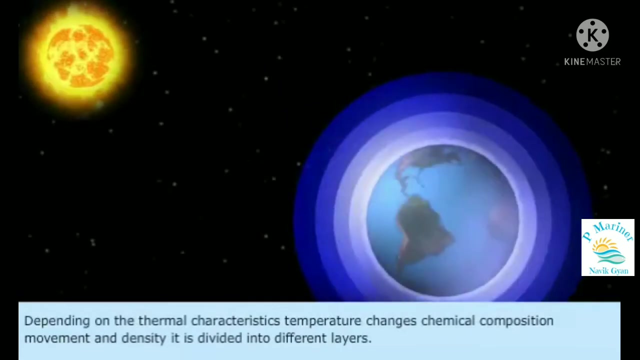 Earth's atmosphere changes from the ground up and is primarily composed of nitrogen- 78%- oxygen 21% and argon 1%. A myriad of other very influential components are also present, which include water, greenhouse gases, carbon dioxide, etc. Depending on the thermal characteristics, temperature changes, chemical composition, movement and density, it is divided into different layers. The ionosphere extends from 80 to 200 km above the Earth's surface atmosphere, and this is the layer of atmosphere that is ionized by solar radiation. The thermosphere is the fourth layer in the atmosphere. Space shuttles fly in this area and it is also where the aurora lights are found. 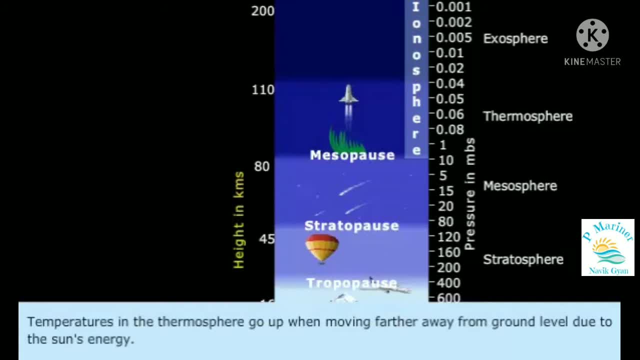 Temperatures in the thermosphere go up when moving further away from ground level due to the sun's energy. The increase in temperature stops at this height, beyond which lies the exosphere. The mesosphere is the third layer. It extends from 50 to 80 km above the Earth's surface. 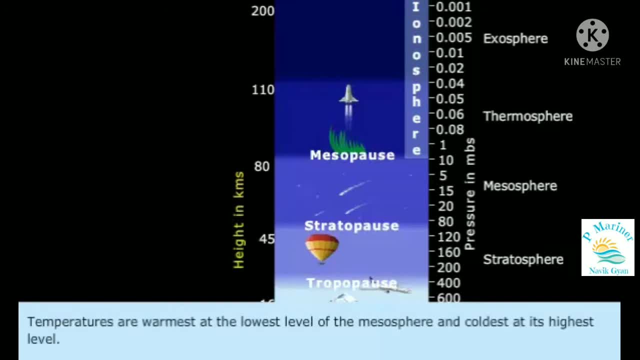 Temperatures are warmest at the lowest level of the mesosphere and coldest at its highest level. The stratosphere is the second layer. The stratosphere is the third layer. It extends to about 45 km above the Earth's surface. 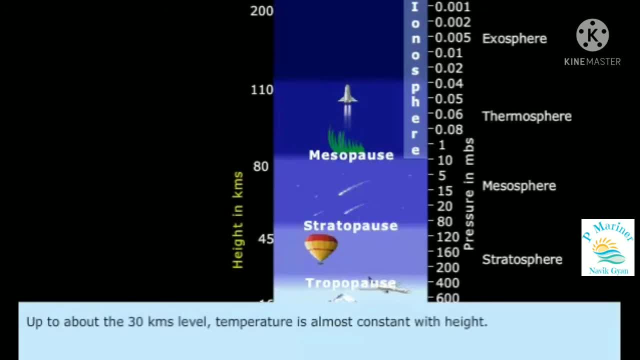 Up to about 30 km level. temperature is almost constant with height. In the upper stratosphere, temperature increases with height. Very little water vapor is present in the stratosphere and this lack of water vapor results in there being no weather. 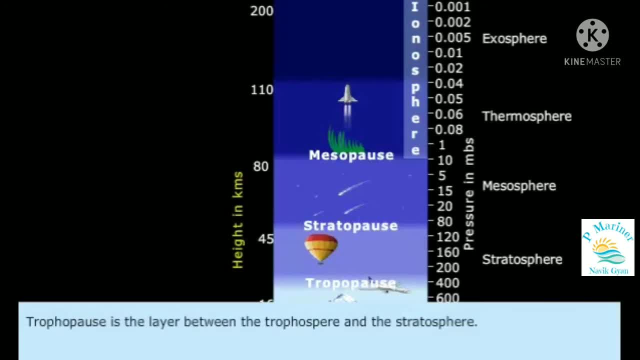 The tropopause is the layer between the troposphere and the stratosphere. The troposphere is the layer closest to the Earth. Whatever happens here is described as weather, because it is this layer that contains most of the water vapor that leads to the formation of clouds, rain, snow or other weather features. 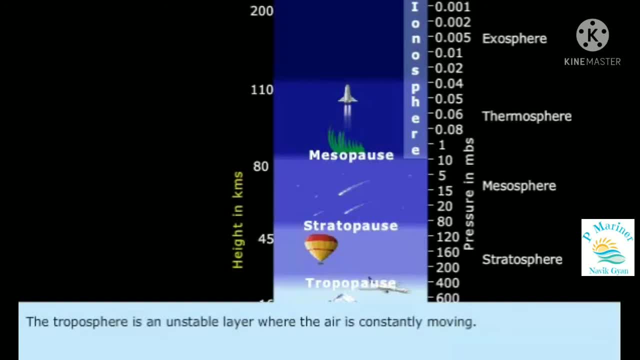 The troposphere is an unstable layer where the air is constantly moving. The thickness of the troposphere varies from about 8 km above the poles to about 16 km above the equator. The chemical composition of dry air is constant within the troposphere and 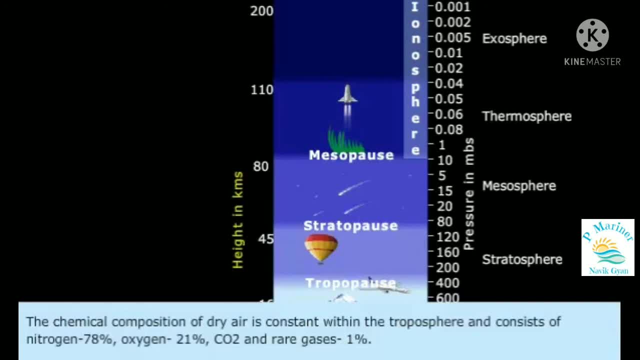 the amount of nitrogen in the troposphere is 78% and the amount of oxygen is 21%, and the amount of carbon dioxide and the amount of rare gases is 1%. Generally, temperature decreases with height within the troposphere. The average rate of decrease is 6 °C per km, but large variations from this value are common.